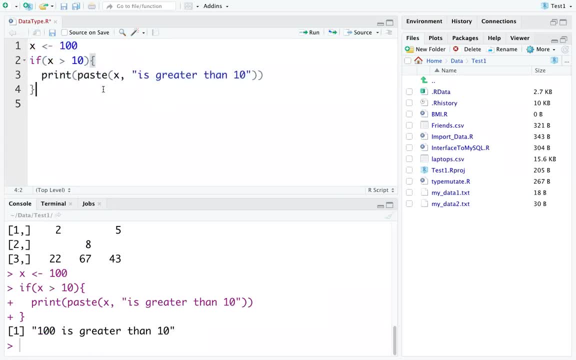 100 is greater than 10.. Now that is fine. Now, if I want to put else part, let's say, if something is there in the input but it is not greater than 10, then if it is, let's. 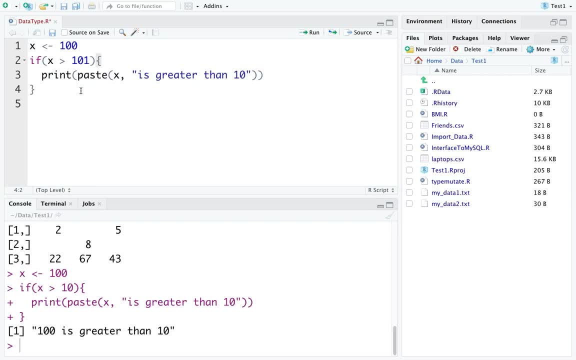 say like that, so definitely it will come in the else part. So else will write just after we are. we are finishing the if statement. So if I'll put like this, then it will be a problem. See, it is unexpected token, else it will not take like this. So 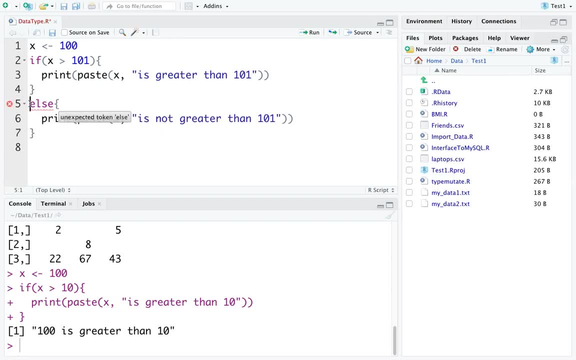 remember if I using, if else it will be like this: Now it is working And it is going to work. So here the else part, it is going to work. 10 is not greater than because we have put it the condition 101. So 100 is not greater. 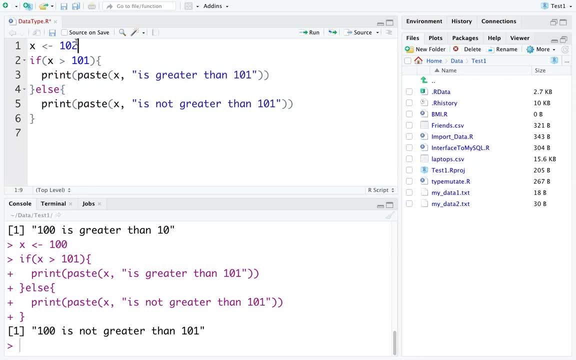 than 101.. I will put it two. So if is going to work, because the condition is satisfied, 102 is greater than 101.. 102 is greater than 101.. This is going to be a problem. So, if, if a statement is the right, if a statement is the right, if it is going to work, then 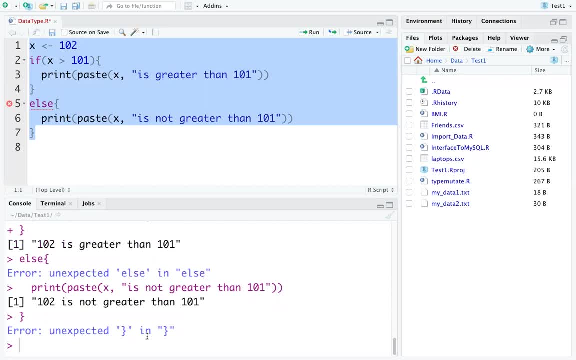 it is going to be better than 101.. This is how your. if a statement is This is not correct, it will give you error or exception. error is giving it. So remember this If you want to put L else. if, Ms Nested, you can do like this: 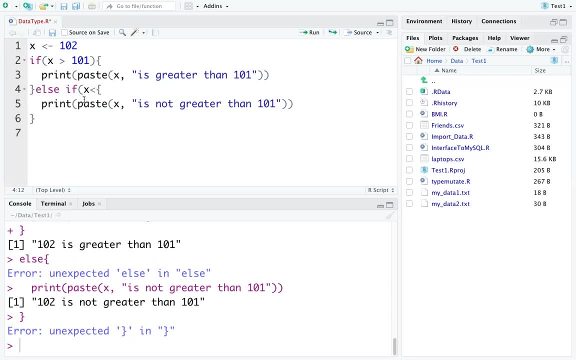 All right, right. so else, if we can use this like this and at last we can write else and we can print elsewhere. now here we have written two conditions, which is definitely as going to satisfy, but if it is there is yeah. so if else is going to work like this, so definitely if it is one, zero one. so first, 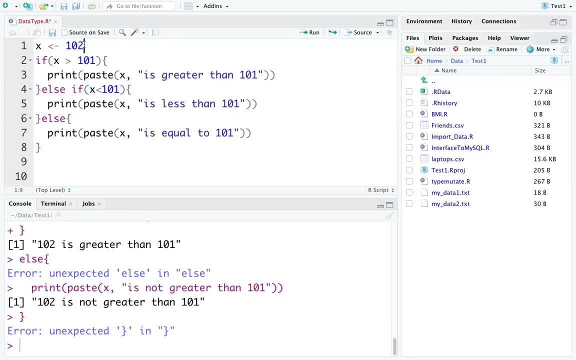 if condition is satisfying. if it is less than that, let us say we'll make it hundred by正 geographical. other than this, I am going to say that if it is more than if condition, so this is going to uh execute the second. if else 100 is less than 101, but if i'll say 101, 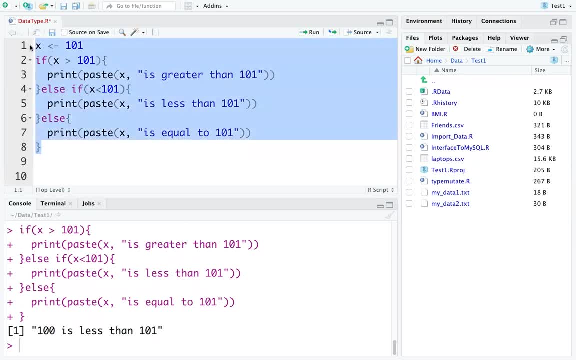 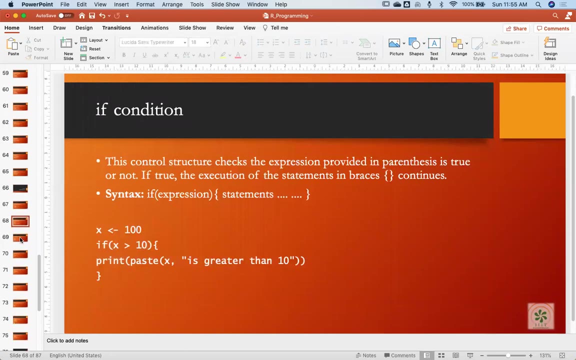 then else part is going to be executed. 101 is equal to 101, like this. so this is your. l is a if else statement. it is very simple way of learning it about the nested if also i told you then there is a for loop. for loop is: 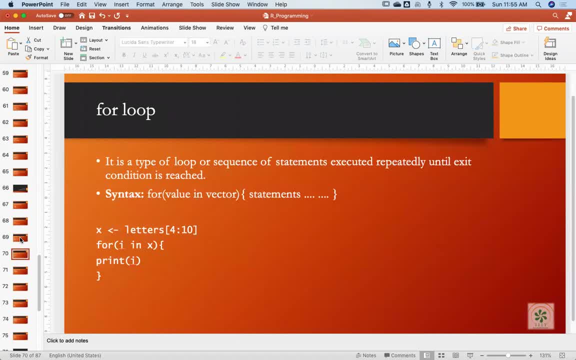 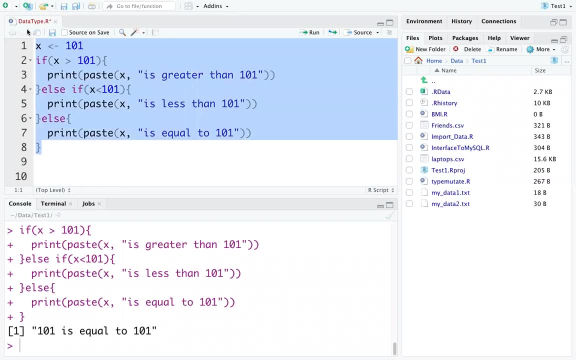 is just similar to what we are using in r. okay, this for loop, the syntax of the for loop, is similar to what we- are sorry- using in python. so python and in the r, the for loop, uh, are almost the same. now here, if you'll see, there is uh. 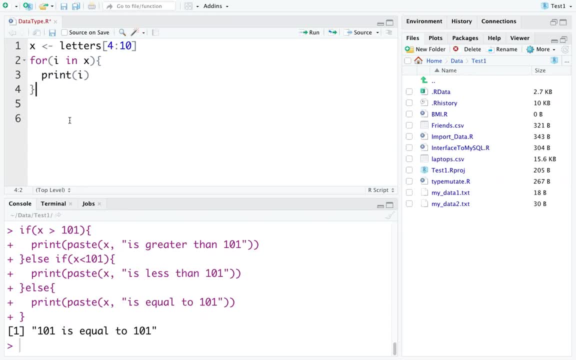 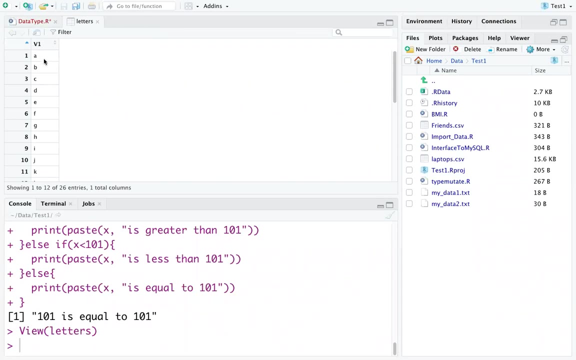 there is a data set called letters. if you want to see this data set, you can see it. this is the data set. here we have the value from a to z, right a to z. all are in the small letter. okay, so this is the data set, which is already there in your base package. so this is there in. 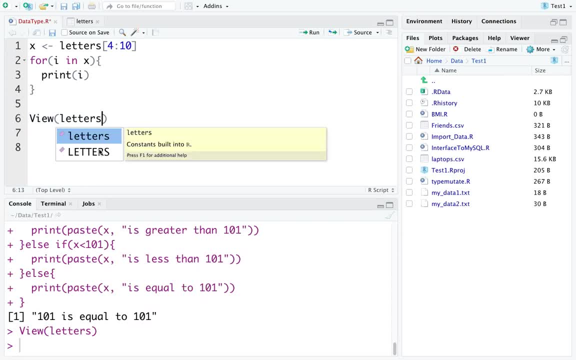 the base base package. okay, letters is there in the base package, as you can see, letters is also there which is having all a to z value in the capital letter. so that letter we are taking and we are taking the value from 4 to 10. 4 to 10 means this: 4, d to j, d to j, and we are printing the value from i in x. so is starting. 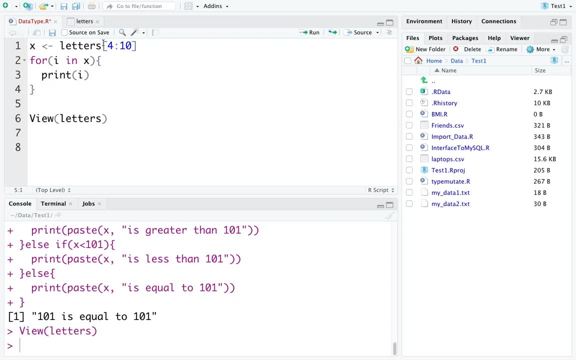 the value is i. i is pointing to the fourth, the first character which is there in 4, which is d, and it will go up to up to what last is last is your j. so 4 to 10 it is taking. i to d to j, it is taking and it is printing it. so let's run this. 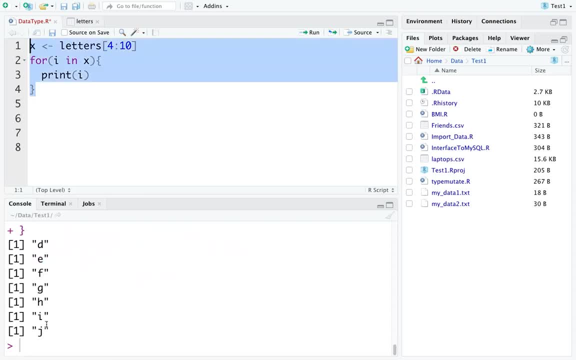 see d to j. it is printing. right, it is taking the value from uh particular. now, if you don't want to do that, you just write it like this: there is a value from 1 to 10 and then it is going to print the value from 1 to 10.. see, it is going to print the. 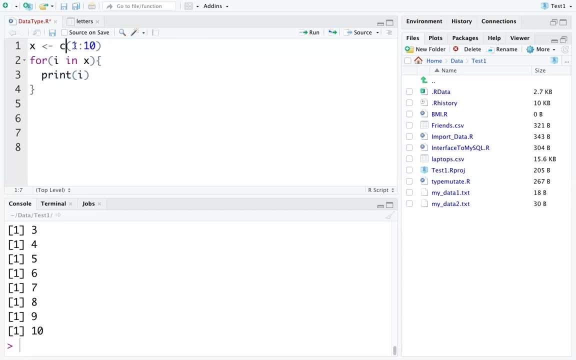 value from 1 to 10.. so here i have created a vector with 1 up to 10, or if you want to give some steps, you can give it. so i want to step at a time. wait a minute. no, no, it is not going to work. 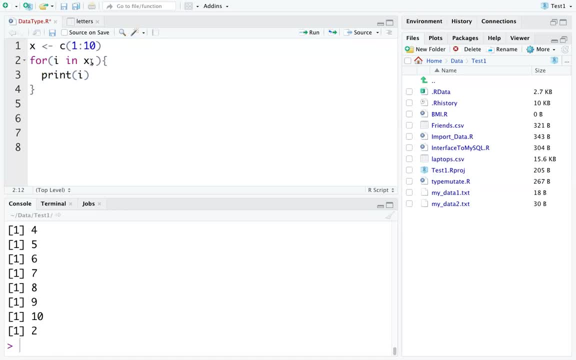 here. let's see it's giving the exception. okay, uh, so this is your for loop. uh, i is pointing to the first one and it is. it is increasing, it's Uh, it's uh, counter one by one, and it is taking the data from x and it is printing the value of i. 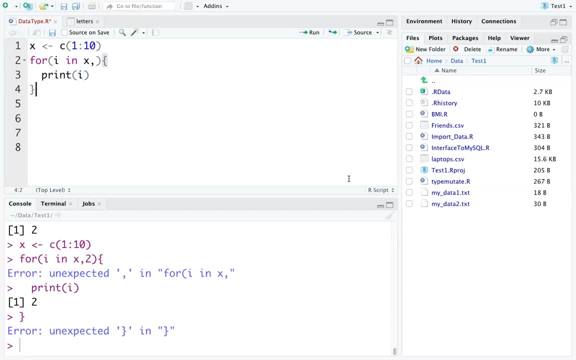 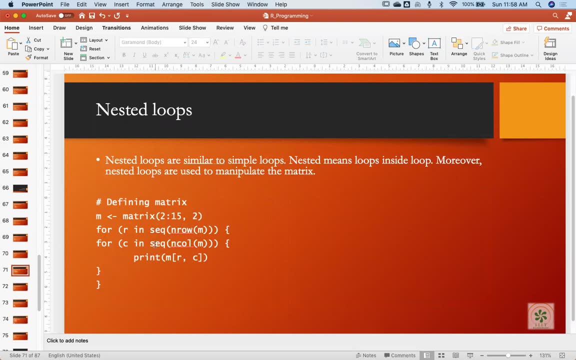 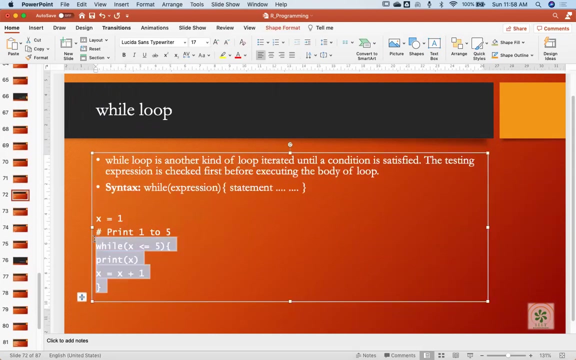 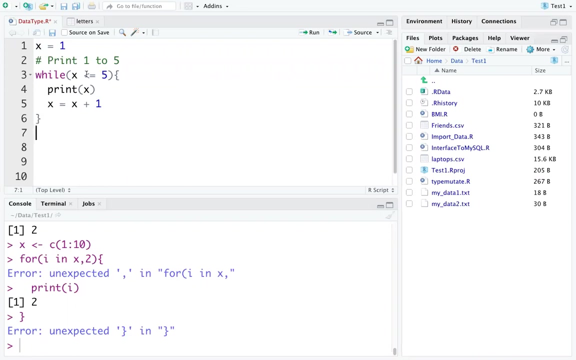 this is the for loop. okay, then we can do for loop for loop inside another for loop. we can make an uh, a nested uh loop for loop inside another for loop, while loop is also there. all right, we know that there is a condition: that to be uh, that need to be if it is satisfying when we are. 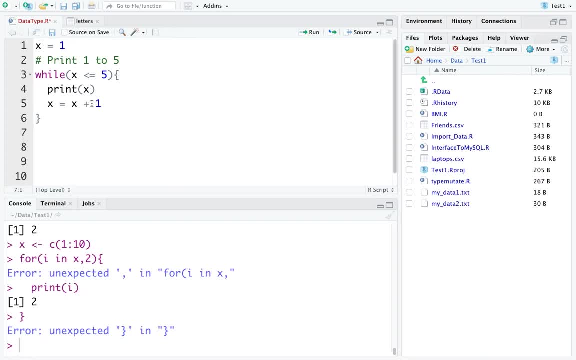 going out. otherwise, sorry, if it is satisfied we are going in, if it is not satisfied, we are going out. so it is saying that x should be less than or equal to 5. if it is x is 6, then we have to get out from that particular loop. so up to 1 and 1 to 5 it is going to print and if it is coming, 6. 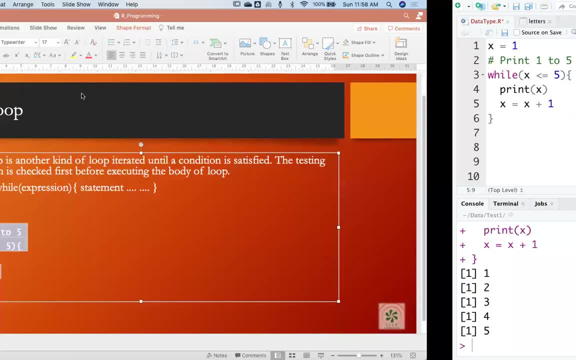 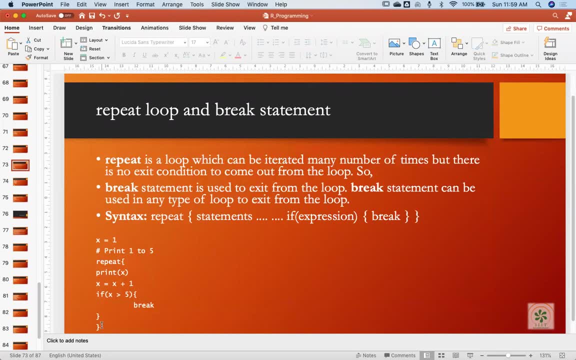 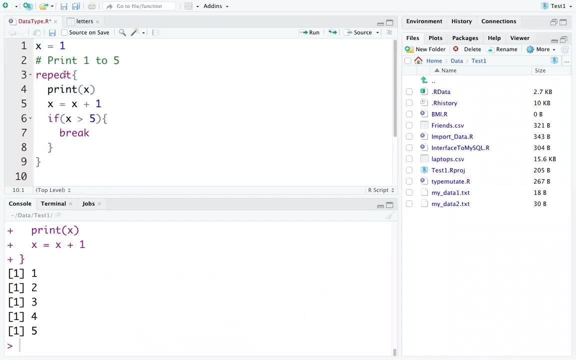 then it is going out. so this is the condition that we need to get out from: that particular loop is your while loop. then there is a repeat. uh is also there in repeat. we does not have any condition. see in repeat, we does not have any condition. instead, we have a break. so if this condition will be there, if x is greater than 5, 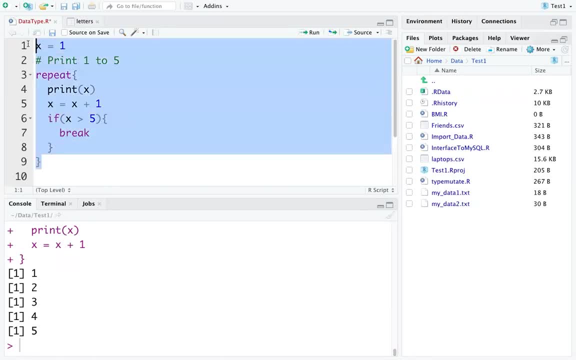 then we have to break right. so this repeat is also a control loop- is taking the value of x is greater than 5 and x is greater than 5 and x is greater than 5, then we have to break so because right now the value of 5, a value of x- is 6. that's why it has been. 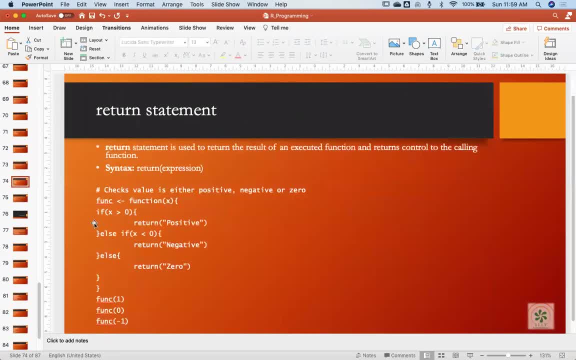 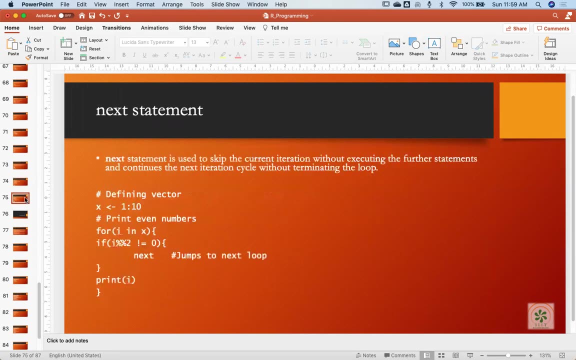 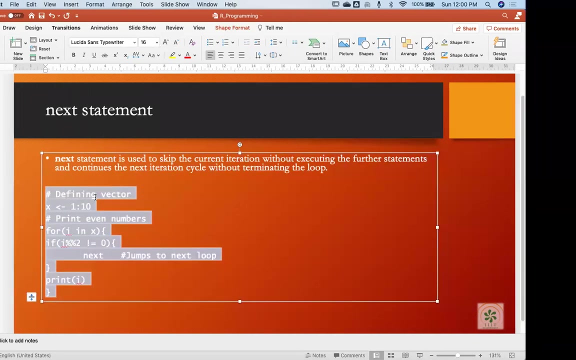 come out from the loop. there are different return x expressions. if we are in the loop and we are saying that something has to be written, then return function has to be written as has to be right, and then there is a next uh statement. this next statement is, uh, not going to break. 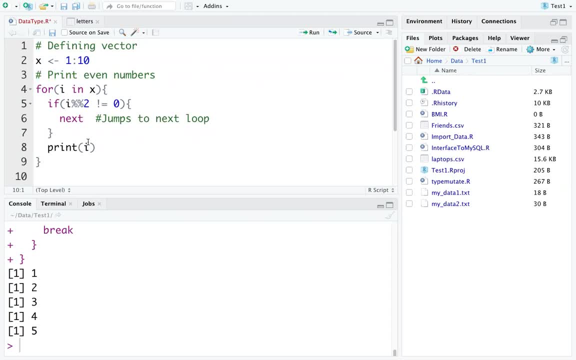 anything, but what if it is coming? we are still in the room loop, but whatever it is, it is there. afterwards it is not going to print, so print statement is not going to work. in the next it will again come to the loop. so here we are in the loop and we are saying that x is greater than 5 and x is greater than 5. 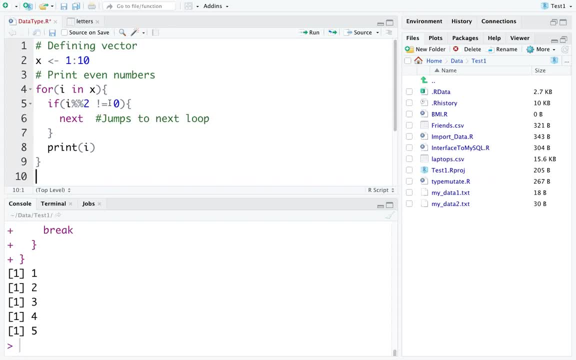 then if you'll see, we are looking for the even number. if it is even number- sorry, odd number- if it is odd number is not going to print. if it is the even number, then it is going to print. so if it is even number, it is going to print. if it is odd number, we are. 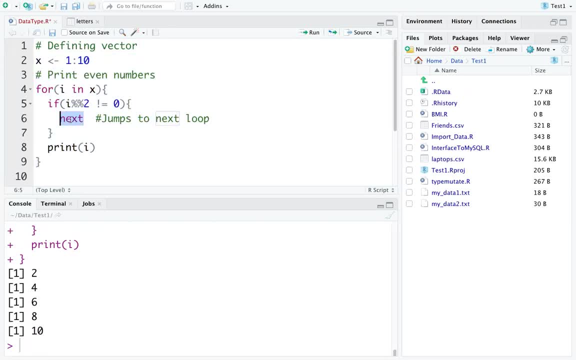 going to the next. next means again for loop will be executed and the i value will be increased by 1.